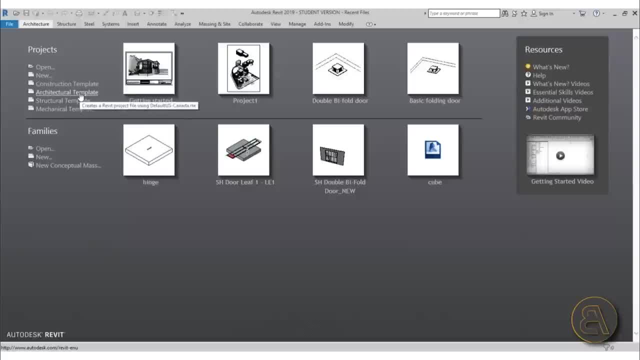 the structural template or you can use the architectural template. it doesn't really matter. I'm just going to choose the structural template and I'm going to use the structural template. and I'm going to choose the structural one because it gives you just some presets that can be. 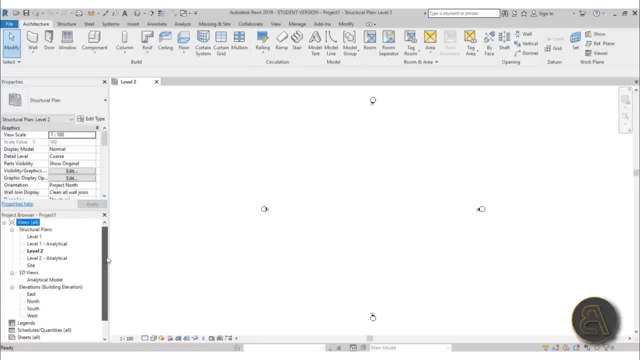 useful. so if I open it up like this, and if you go you can see you've got your levels, and if you go to South elevation, yeah, so you've got some analysis levels. it's not really something that I'm going to be using in this tutorial, but it's. 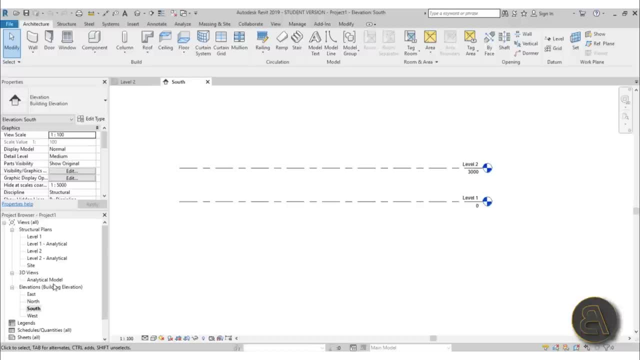 just good to know. you have those and we've got this analytical model and I'm just going to be showing you that a bit later on. so let's go first to maybe a level one and let's create a grid for our simple building. so for that, just go here to grid or you can use 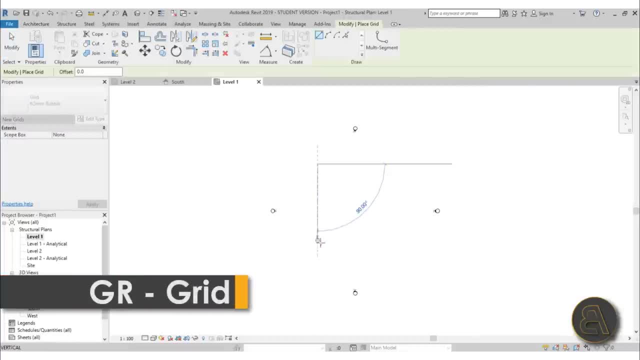 the shortcut gr is the shortcut for grid, and then maybe just do one line like so, and then you can just use the offset. so again, I'm just going to type in: gr for grid, use the offset tool, give it an offset of, like I don't know, six thousand. 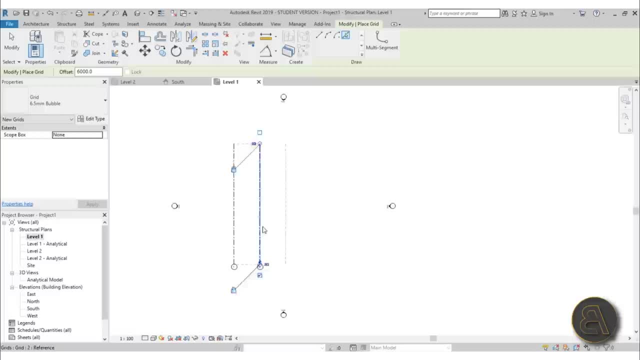 millimeters or six meters. so just go like that and let's make something simple like: so. then go again gr for grid and do one like this and then again use pick lines. but before that I'm just going to rename this from five to a. and once you do that, when I go gr and pick lines and 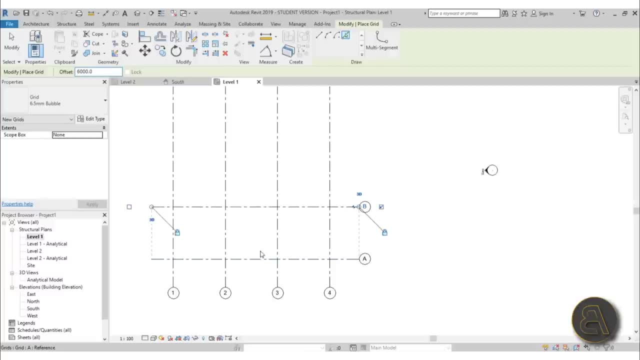 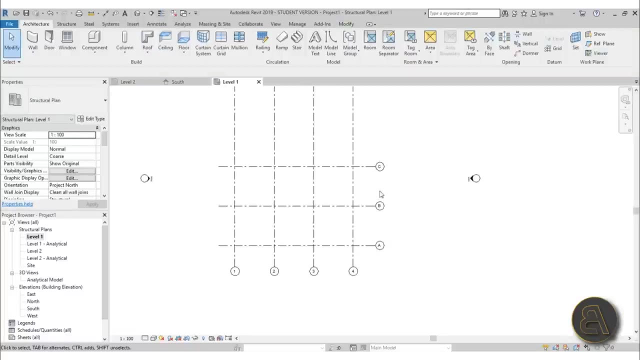 again six thousand, and when I go like this, as you can see now it's going to continue on ABC. so we've got one, two, three, four. one two, three, four and then ABC, and, as working in millimeters is really annoying when you're working in like construction, out with construction, 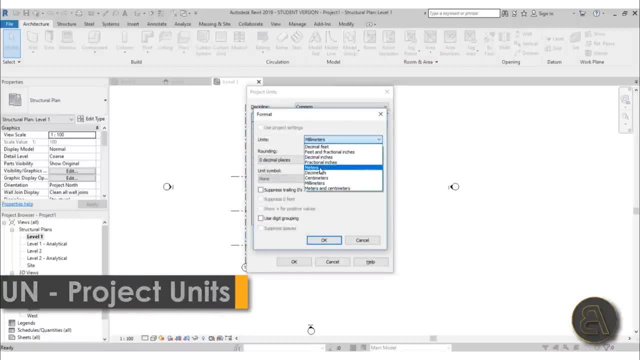 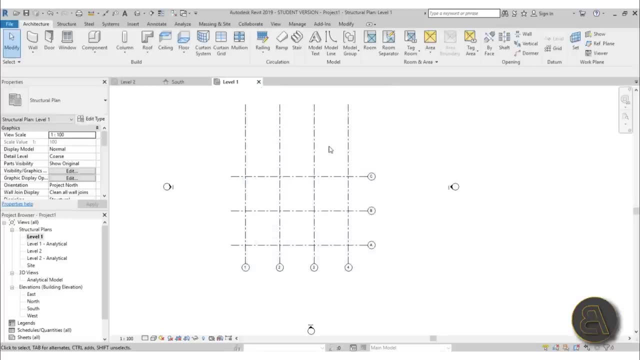 elements. I'm just going to type in UN and change the units to meters and give it to decimal places so we can just see the dimensions or just input them a bit easier. then I'm just going to select this: get this ring, bring it in a bit. 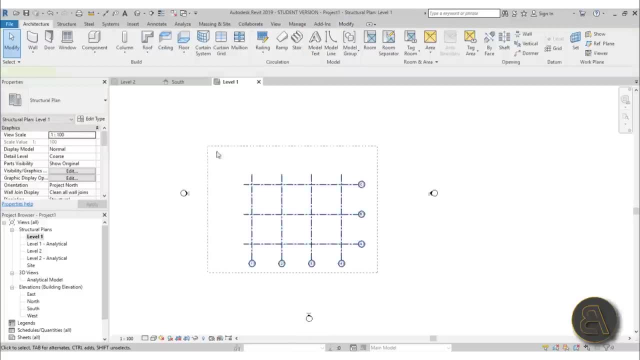 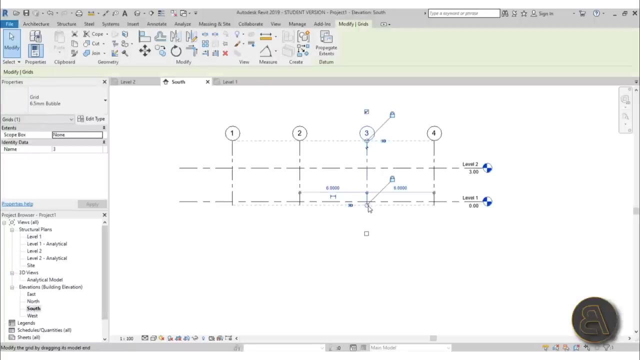 just to make everything a bit better and let's select everything and Center it over here. yeah, maybe that. yeah, that looks good, okay, so once we've got this grid system and now it's time to start adding elements, but before that, I'm just going to go here to south elevation and add one more element, so I'm going to 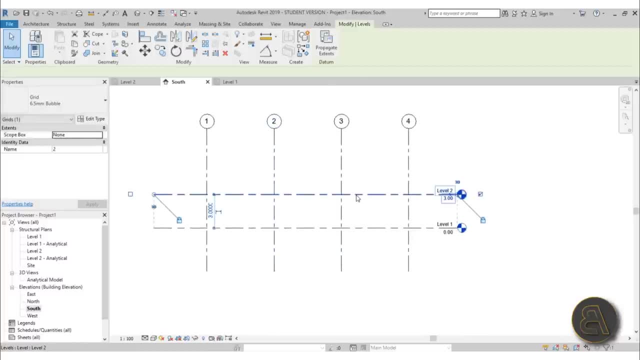 drop this a bit, drop this up a bit, and yeah, let's add another level. so LL is the shortcut for that. and yeah, let's do it at four meters as well. so this is level three, and then I'm going to do one more over here at I don't know something. 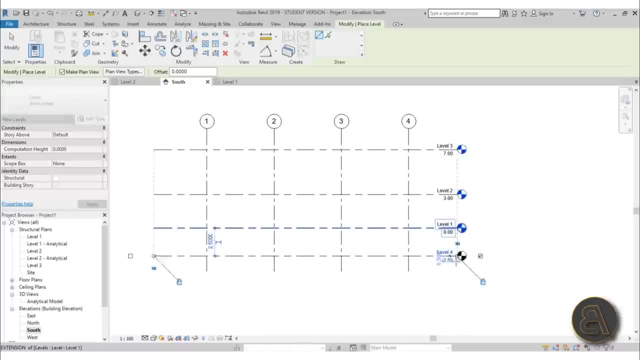 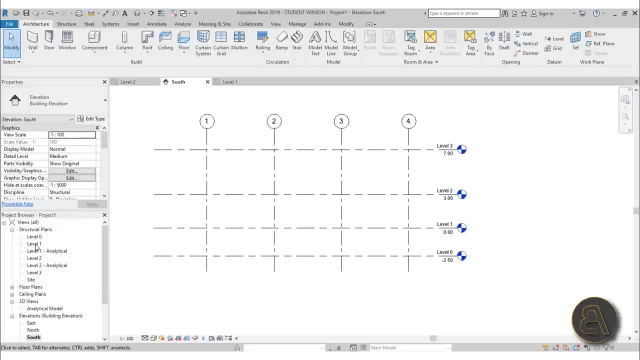 like, yeah, let's do 2.5 and this won't be a level four, this is level zero. so this is like the foundation. okay, so once we have this, now we have all the necessary infrastructure so we can continue or start modeling our construction. so go to level one and here 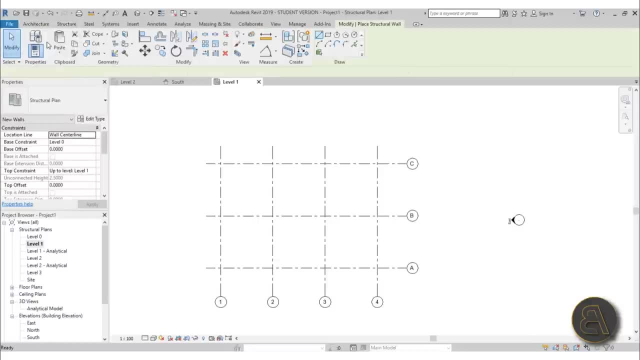 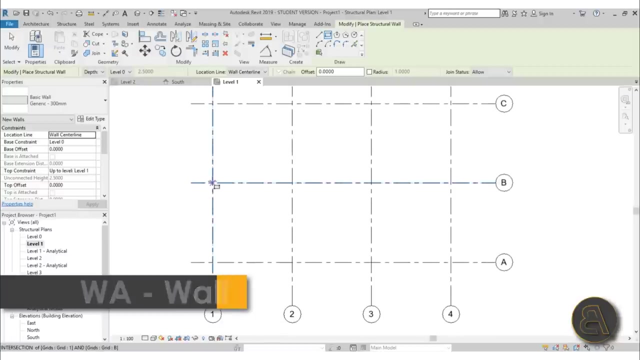 you can go to structure and create a structural wall. so for the structural wall, let's go with something like a generic 300 millimeter, and this is for our structural core. so I'm just going to go here with a rectangle and then select one of these quadrants and let's go with here and go from here to here. and then I'll select one of these quadrants and let's go with here and go from here to here. now 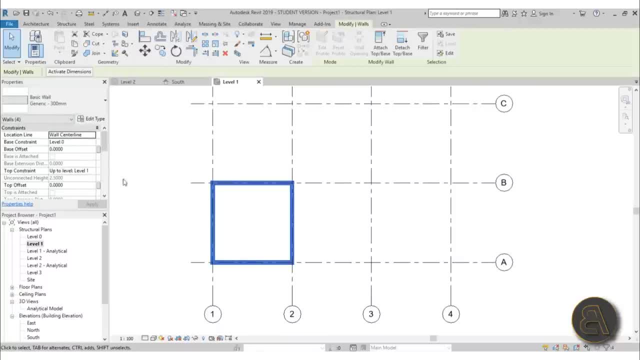 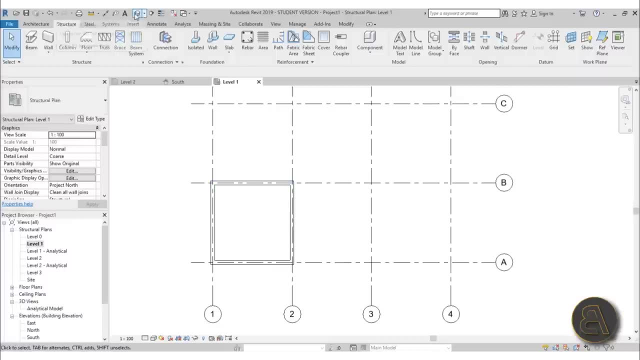 Now I'm just going to hover over one of them. hit the tab key, select all of them And then base constraints should be at zero and the top constraint should be at level three. Okay, So once we have that, let's go into 3D. 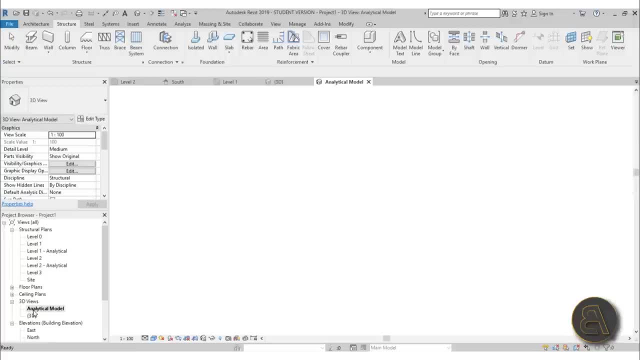 Yeah, this is what we want And, as you can see, this is that analytical file. So if you go to analytical mode, you can see this is just a graphical representation of the analytical model. So this is just calculating your walls as far as structural elements go. 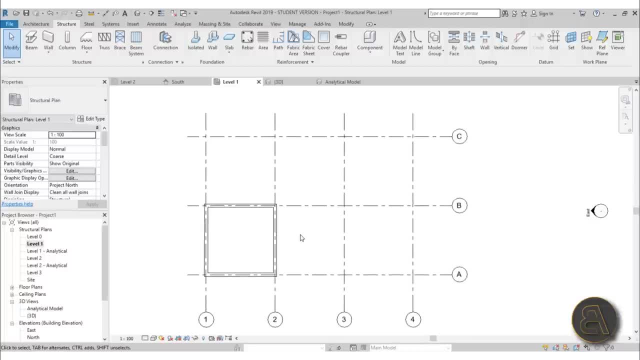 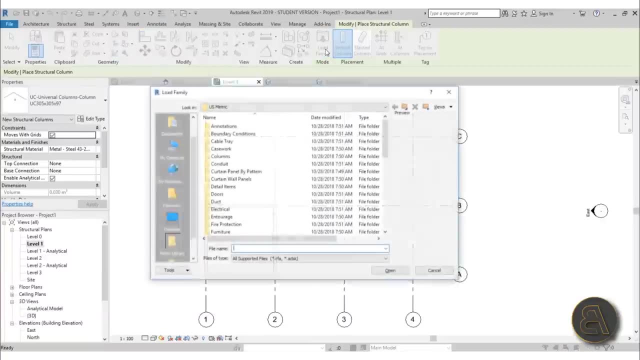 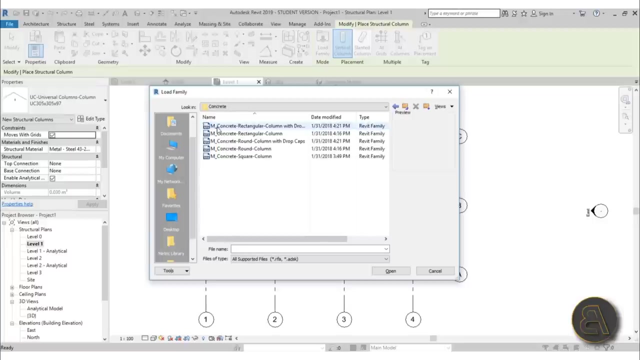 Okay, Let's go back into level one and let's add some columns. So go here to structural column and let's just load in a family, because we only got to this steel columns and I want to use some concrete ones. So I'm just going to scroll down to structural columns. go with concrete and we've got square. 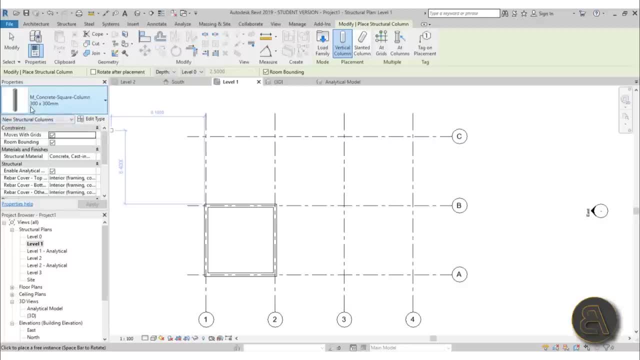 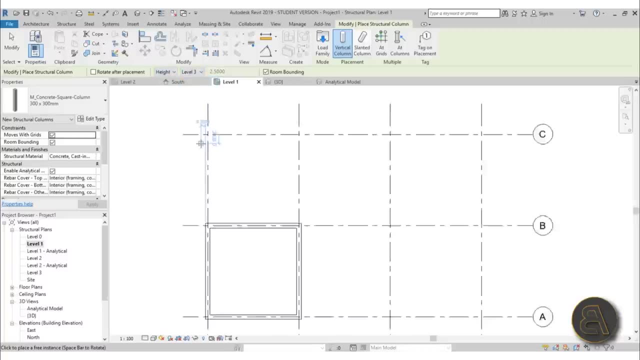 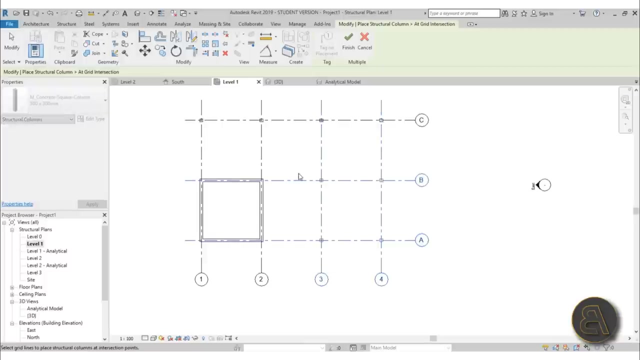 concrete. Open that up, Okay. So I'm going to choose this one, 300 by 300, as this is a small building, and let's give it a height to level three, and then just put one at each intersection of these grids, or you can use at the grids and then select like this and go finish. 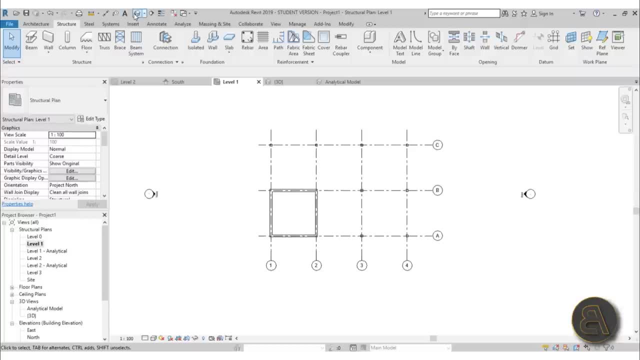 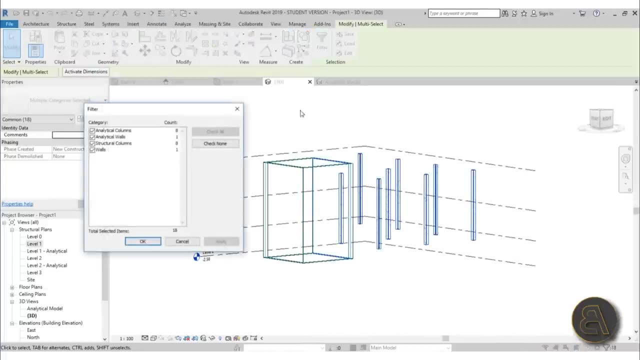 And, as you can see now it's placed them all the way there. Okay, So now if I go into 3D, as you can see these don't really go up to foundation, So I can select it like this: Go to filter. 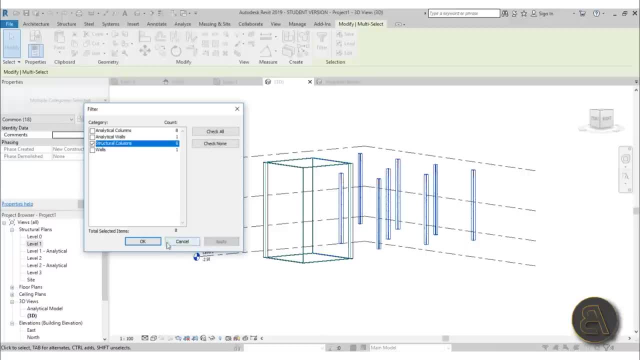 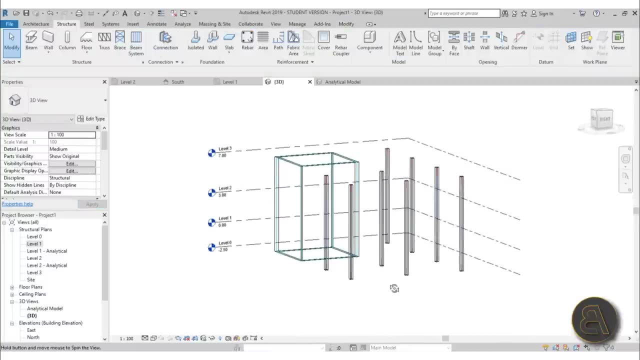 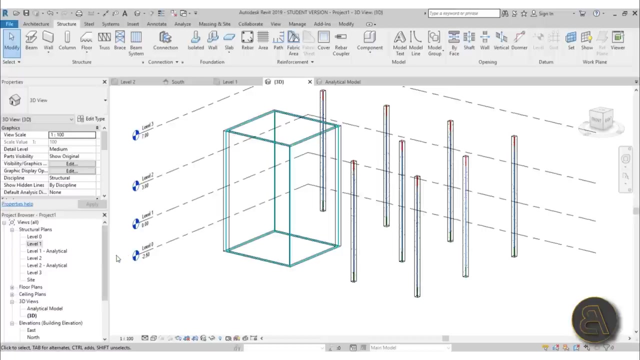 Check. none Go with. structural columns Apply- Okay, And then move them to level zero as well- Okay. And as you can see now, they go all the way up to foundation- Okay. So once we have this, let's add our structural beams. 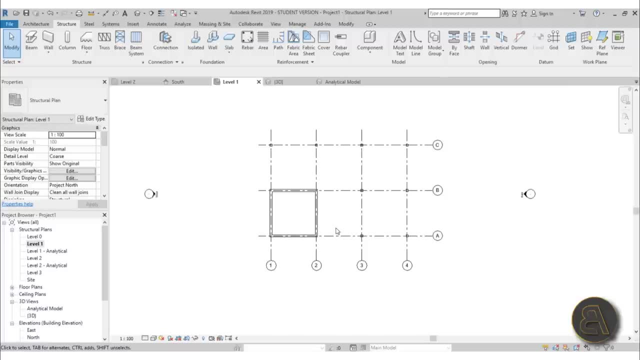 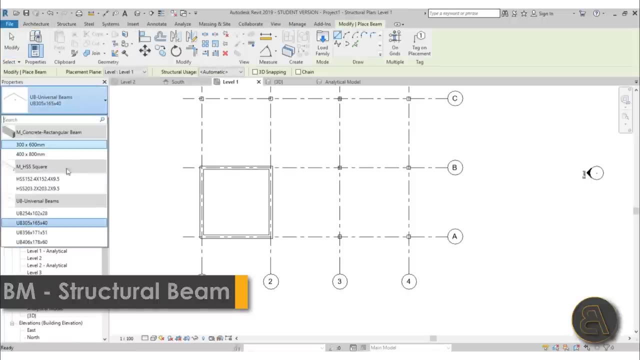 So for beams, you go back into level one and let's go. So we go here to beam and again we only have a steel, Okay. No, we've got some concrete beams. Yeah, That's why I chose the template, the structural template, because you've got some preloaded. 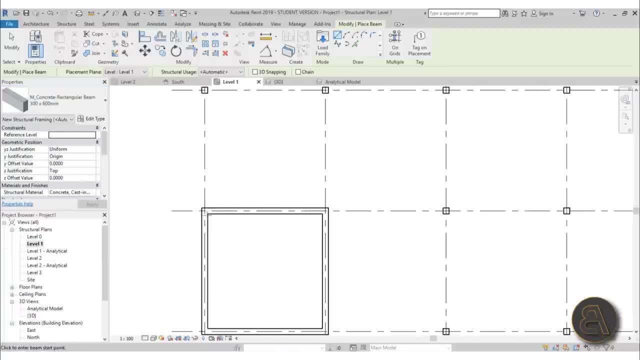 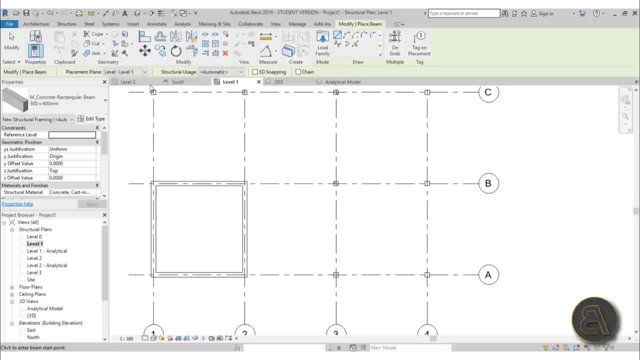 elements. So just go with the beam and then you're going to have these like structural beams going one direction, and then you're going to have not one direction, the band one direction and just going to go in one direction, And then we're going to have some structural beam system going in another direction. 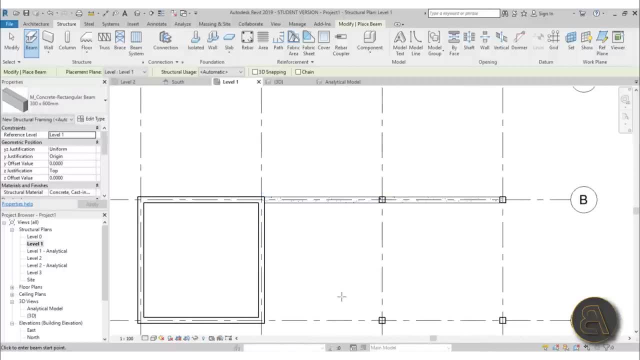 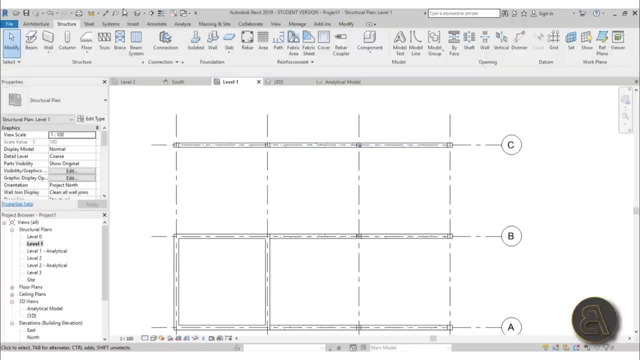 So maybe go from here, from this point, all the way to this column. Then you go from this column all the way to this column and here add one like this: Okay, So once we have this, let's go into 3D. 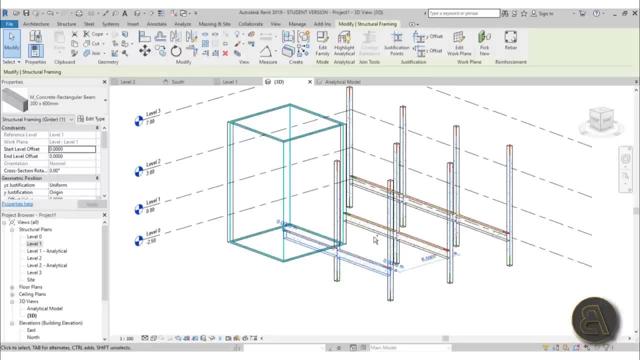 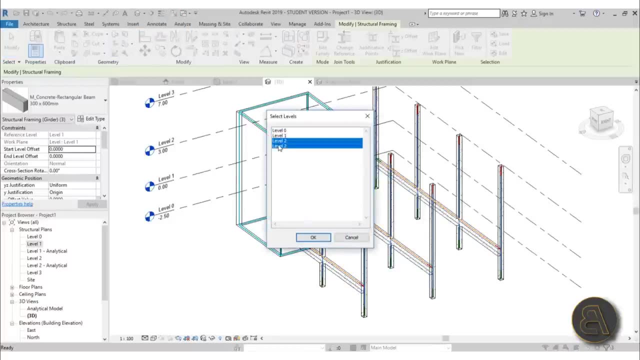 Yeah, I really like the way this is turning out. So now I'm just going to select all of these three, Go here to copy paste, align to selected levels and go to level two and three, hit okay And there you go. 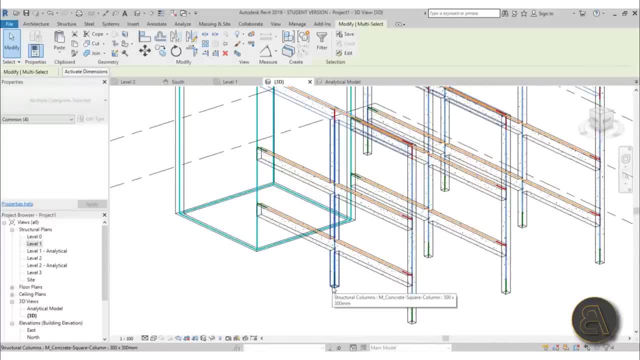 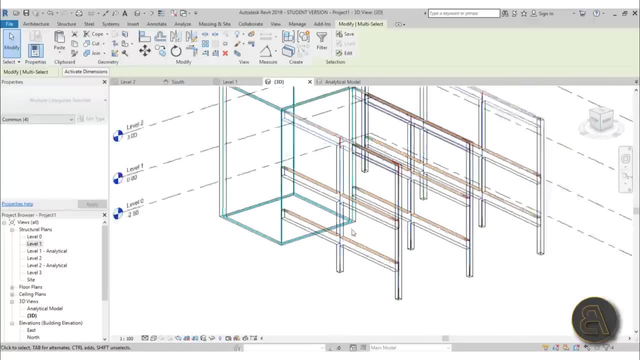 So now this is at all levels. Now, sometimes you're going to have them at foundation, sometimes not, depends on your foundation system. So for now on, I'm just going to leave it without the beams, but if your project requires them, just add. 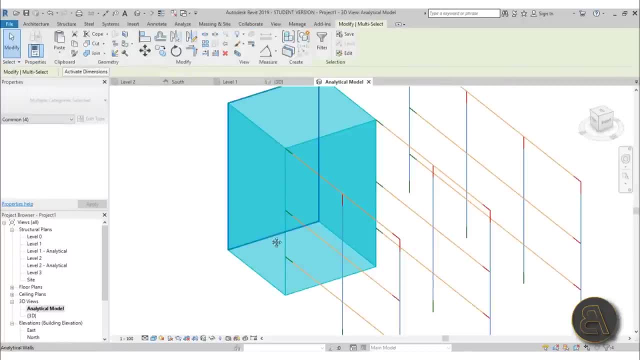 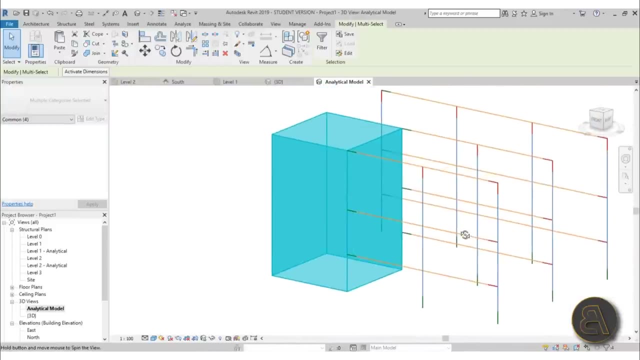 beams. And if I go here to the analytical model, you can see we're already getting an analytical model for this over here. So it's just connecting all of the beams and later on you can send this to somebody doing calculations in robot or something and they can use this model. 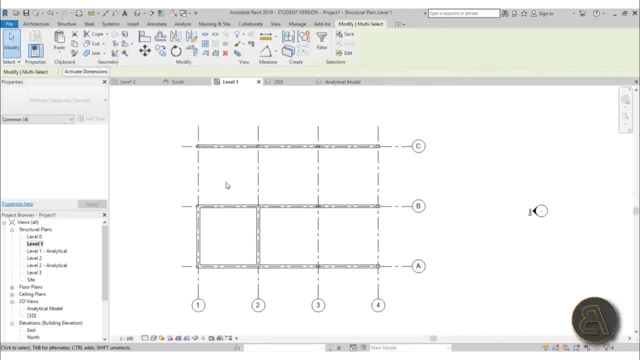 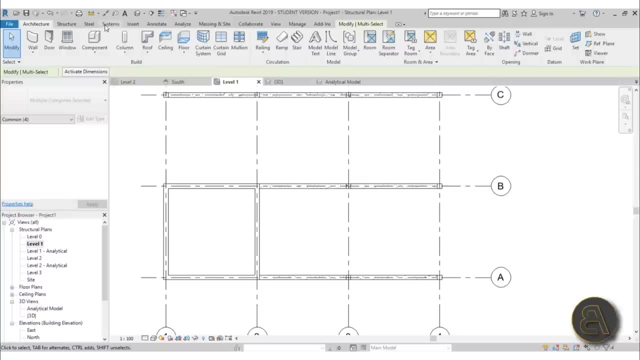 Okay, Let's go back into level one and let's just add that beam system to kind of complete the whole look. And for that I'll just go Here to structure, go to beam system and here you've got automatic beam system or beam system. 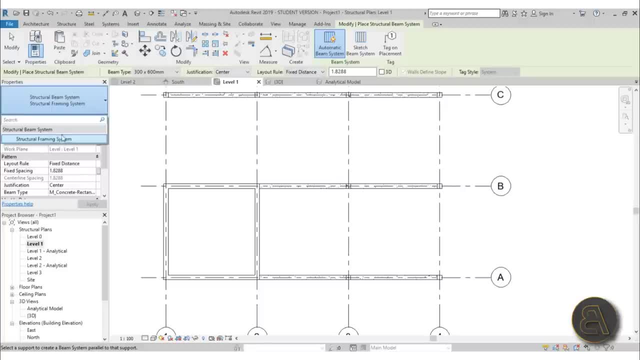 by sketch. I'm just going to choose by sketch. But first when you open this up you can see we've got some the beam type And if we open this up we only have those that are offered as beams, but these don't. 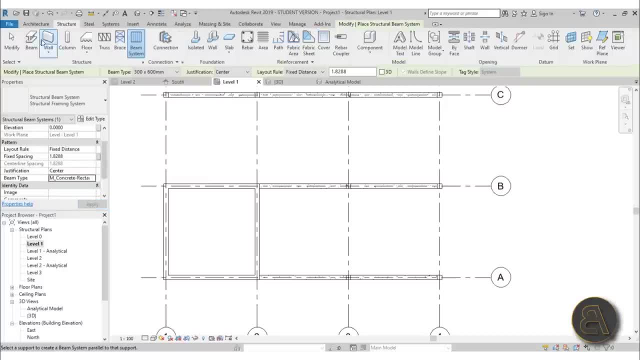 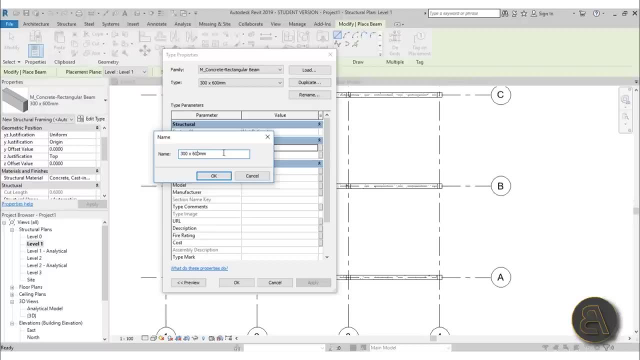 work for our model. They're too, they're too big. So let's go to structure, go to beam and go into edit type and here just duplicate it And let's just call it- I don't know- 400 by 150 by 400.. 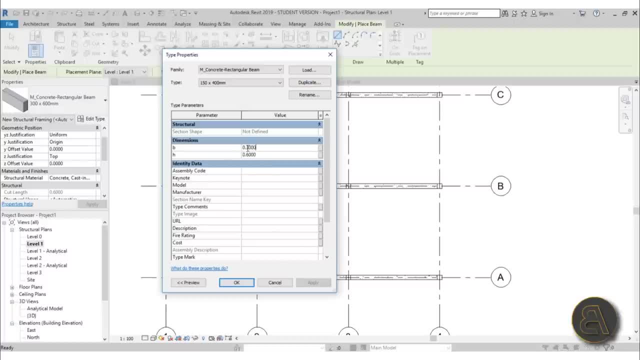 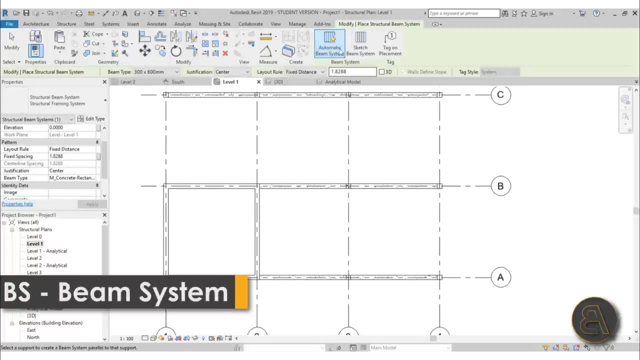 Let's say that works. So hit okay and change this to 0.15 and this to 0.4.. Okay, So once we have this hit, okay. So we've got this smaller beam and now go to structure a beam system, a sketch beam. 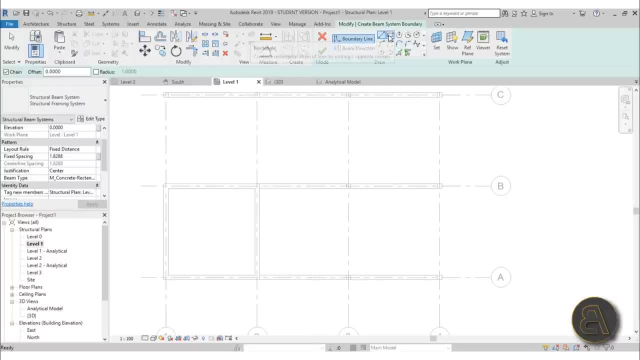 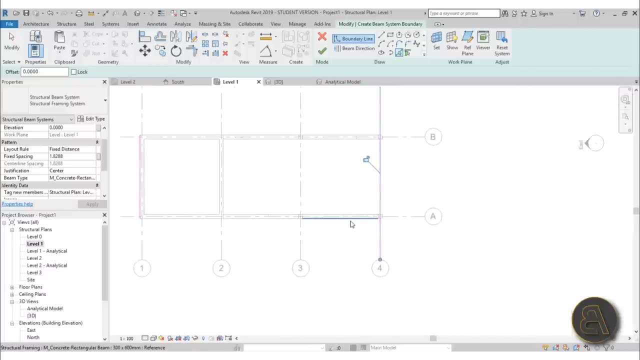 system. I'm just going to go with either pick lines or you can use rectangles. I'm just going to go with pick lines. go from this grid to this end point, over here to this end point, to this end point and just all the way around this wall, but just move. 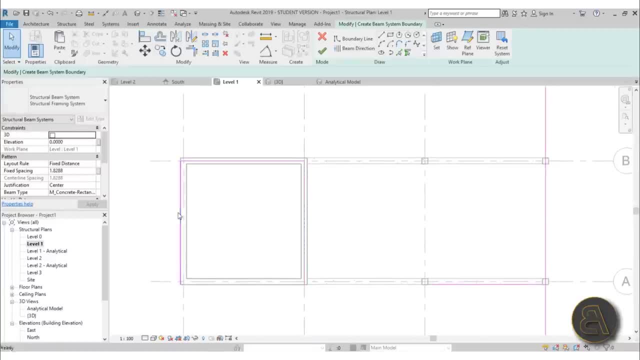 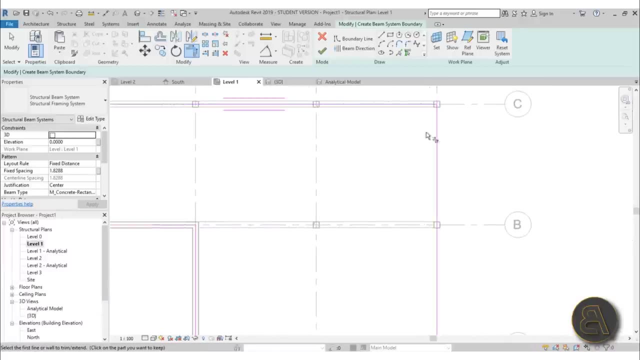 it to grids So those structural elements align, Okay. So now just trim and extend. So trim and extend this, this here, this here, this here and this here, Okay, And move this to the outside of the wall. And if you can't adjust it, just go AL for a line and yeah, do it like that. 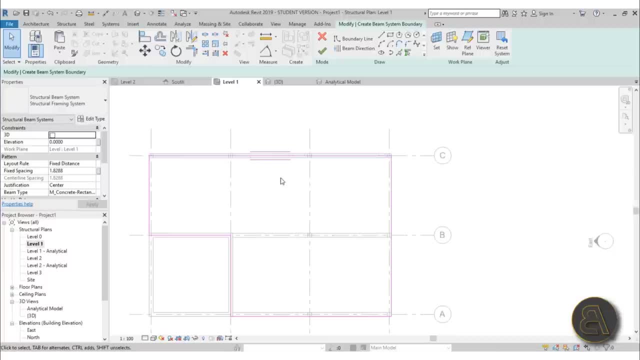 Okay, And this line over here that has these two lines on top and on bottom. that means that's the beam direction, but we actually want the beam direction to be going vertically. So just go here to beam direction and place one line like this: 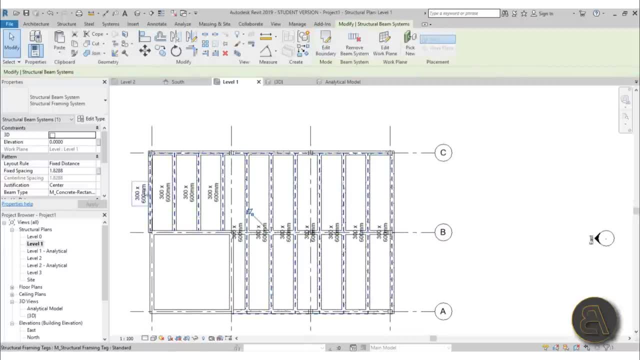 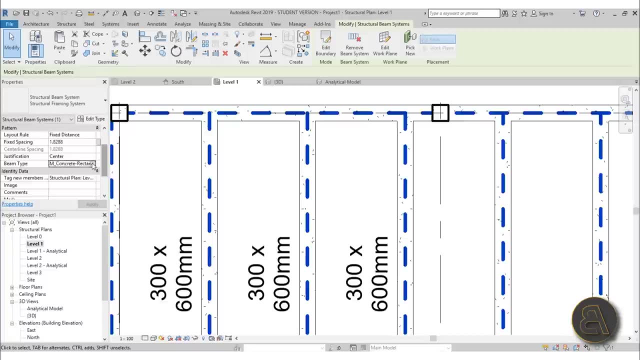 Okay, So just go finish and this is what you get. So now it's the wrong beam type. As you can see, these beams are quite thick, So let's scroll down over here and for the beam type, let's change it to the new, smaller. 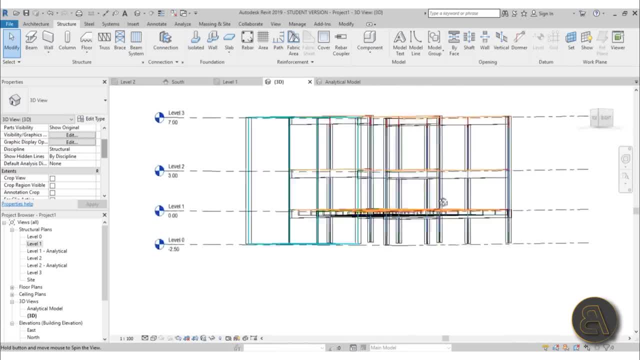 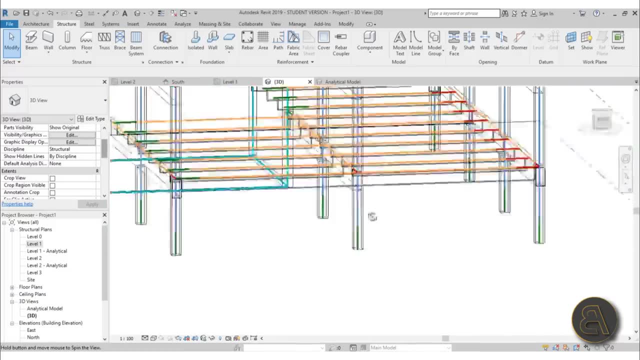 one we have, And now they're smaller. So if we go into 3D, this is what we get. So you can see these are a lot smaller than our big beams going in that direction. So if we look like this, yeah, this actually looks quite all right. 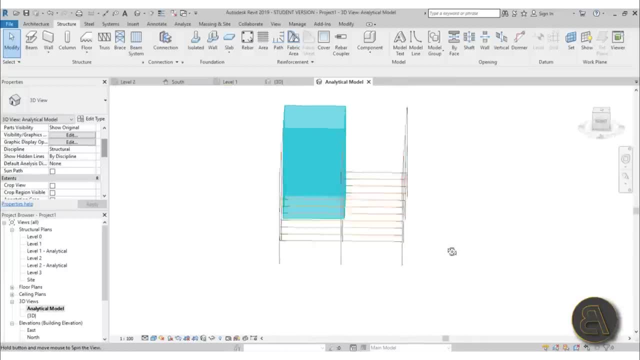 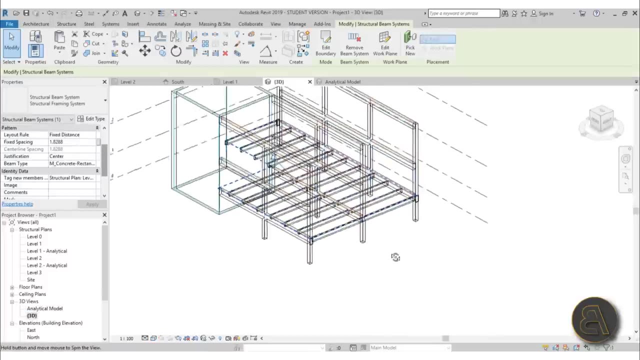 And if we go to the analytical model? yeah, this is what analytical model looks like. So you can go into 3D Hit tab a couple of times, Select the whole beam system and just go here to copy paste. align to selected levels. 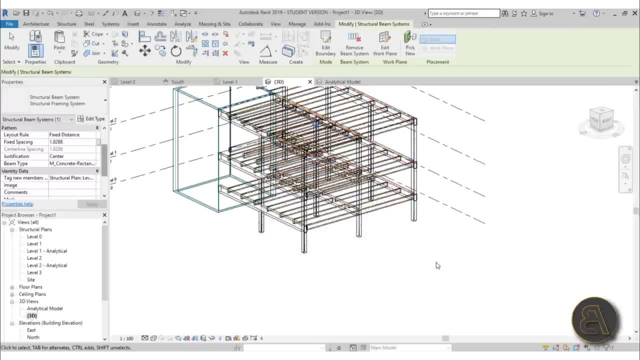 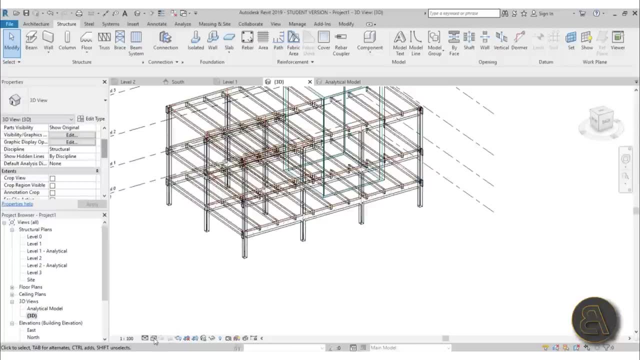 and align them to levels two and three. And there you go, And let's just add some foundation elements just for the fun of it. So, and before that, let's turn this into hidden line, just to see the better, and maybe add some shadows. 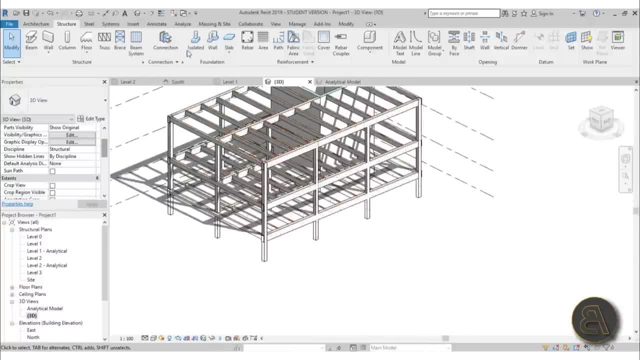 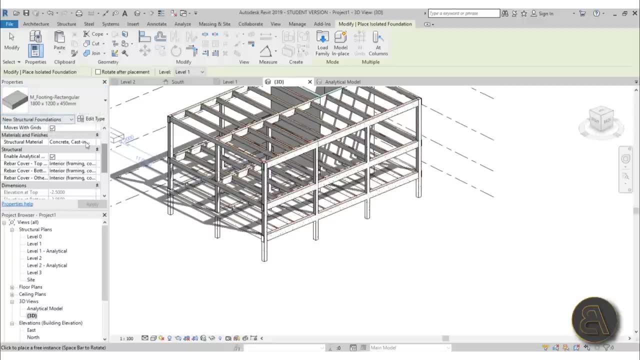 Yeah, That looks cool. Okay, So let's just add the foundation. So go to isolated foundation. And yeah, Let's start with this one. So you're just going to go to level zero And yeah, let's go to level zero. 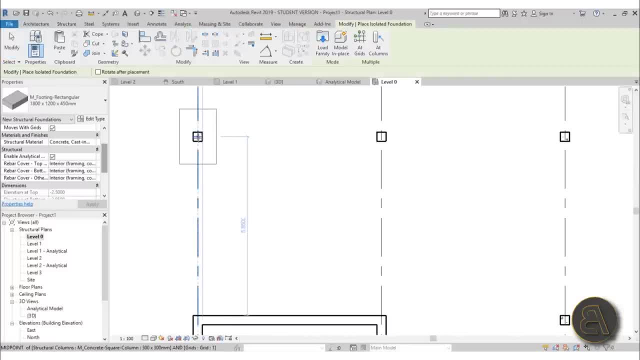 Yeah, This is going to be a bit easier to place it here, And then you place it at all of the intersections, So you go just like that. Okay, I think I missed over here. Yeah, Let's delete that one. So let's place it here, here and here. 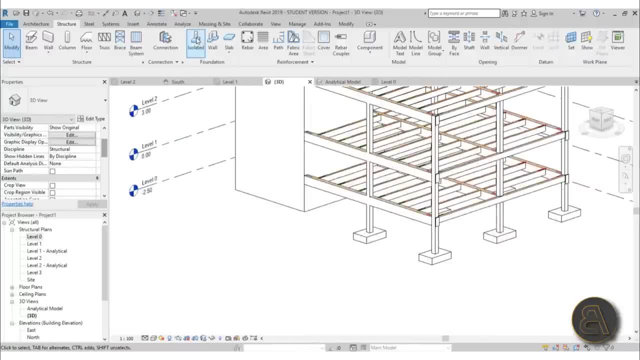 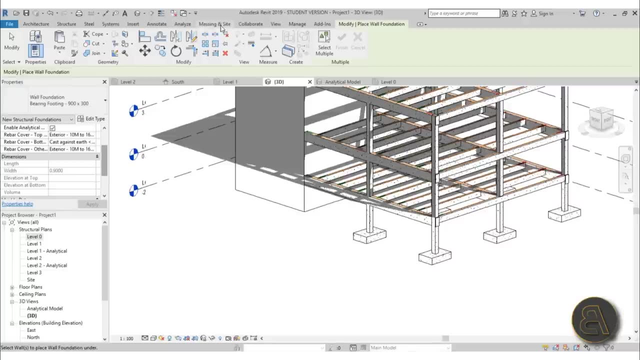 And for our structural core, Let's go. Let's go with our wall foundation, Go, select multiple And then, oops, Let's go back. Sorry about this Wall. Okay, I can work with with the bearing wall, Yeah. 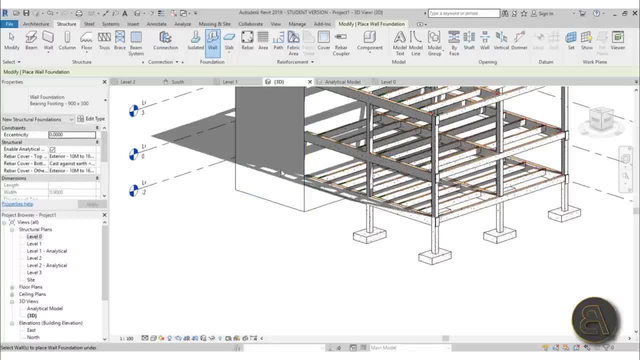 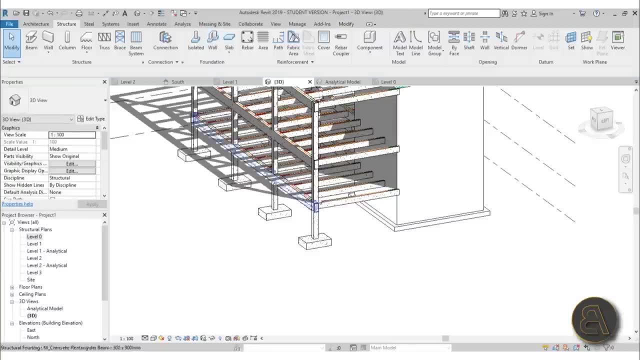 And let's select the. okay, this works. And there you go. So just go all the way around And you place this foundation. Okay, And if we go down, this is where our foundation Lies. And if we go to the analytical model, this is how that thing looks like. 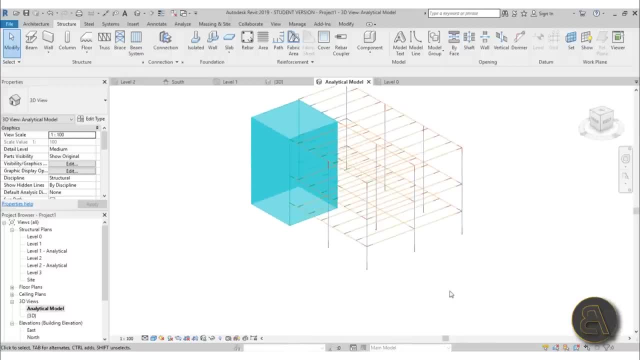 So you can send this to your structural engineers and they can calculate this building construction. Okay, So this is cool. I think you have learned something new about these structural systems and structural elements in Revit. That's pretty much it for this tutorial.